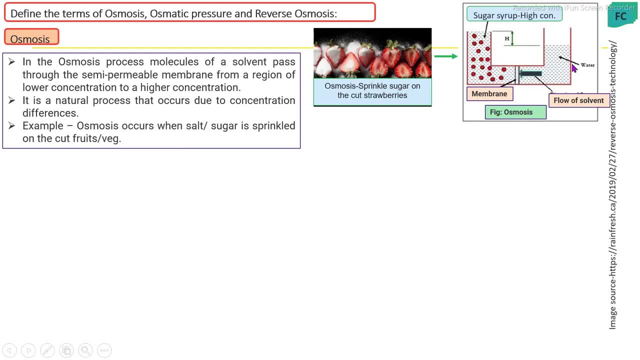 The semi permeable membrane, which is the divided tank, into the two region: The first region, which is the filled with the high concentration syrup or high concentration in liquid, and the second region, this is the water. In this case, water, that means the low concentration solution and this is the syrup that is the high concentration solution. 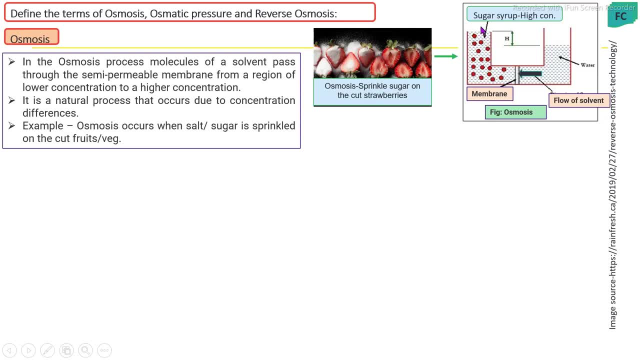 When external pressure, that is, the atmospheric pressure on the both sides, in this case due to the concentration difference there, osmosis process is occurred. That means water, which is the flowing from water phase to syrup phase. that means flowing of solvent from low concentration to high concentration. 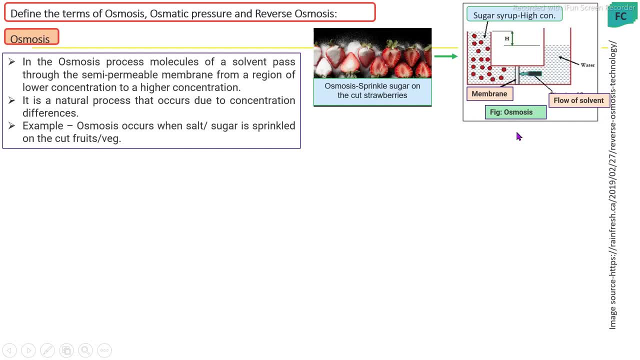 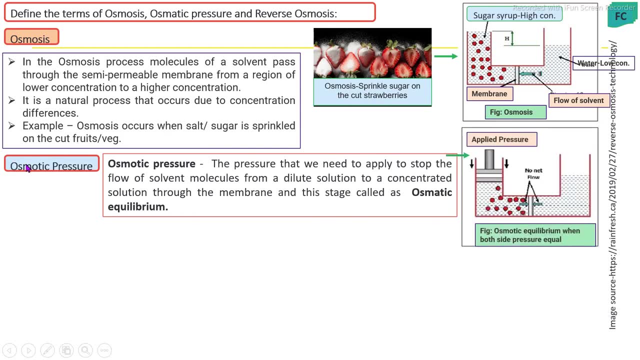 This process is called as osmosis process. Then second point, osmotic pressure. This osmotic pressure is related directly to the proportion to the fruit juice, its concentration, that means its containing constitutes. related Osmotic pressure of the different fruits is vary with respect to the its chemical composition. 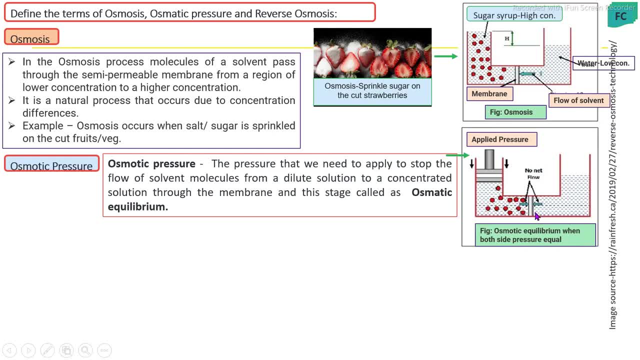 You can see in this example, osmotic pressure. the same image In this process. when we apply the external pressure on the top of the high concentration solution, of the high concentration syrup, This pressure resists to the moment of the water flowing from water phase to the syrup phase. If this pressure completely. 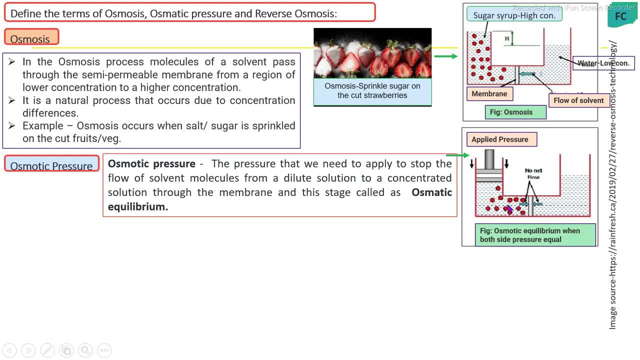 stop the movement of the water flowing from the water phase to the syrup phase. this pressure required to stopping the movement of the flowing of the solvent from the water phase to the syrup phase. This pressure is called as a osmotic pressure. this osmotic pressure occurred when the pressure same. that is the 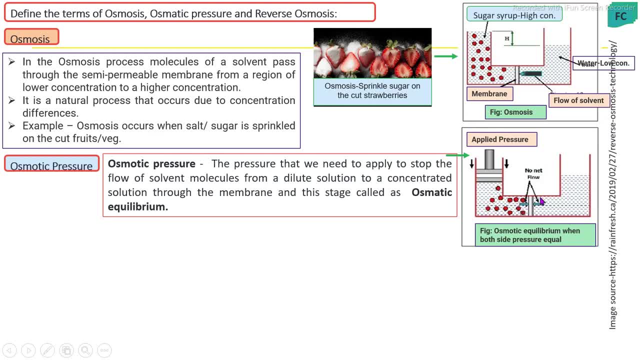 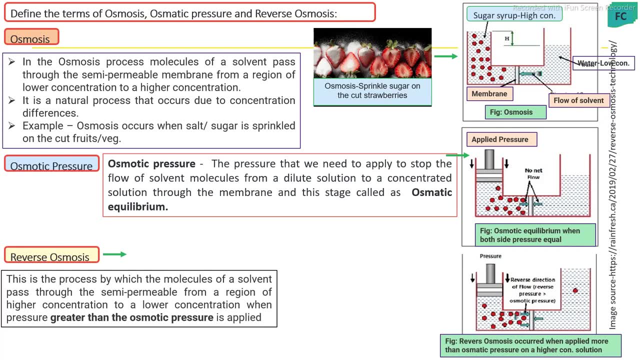 external pressure and the pressure existed due to the concentration difference is called as the osmotic equilibrium process. in the reverse osmosis process, we must require to apply the pressure more than the osmotic pressure. in this reverse osmosis process, when we apply the pressure more than the 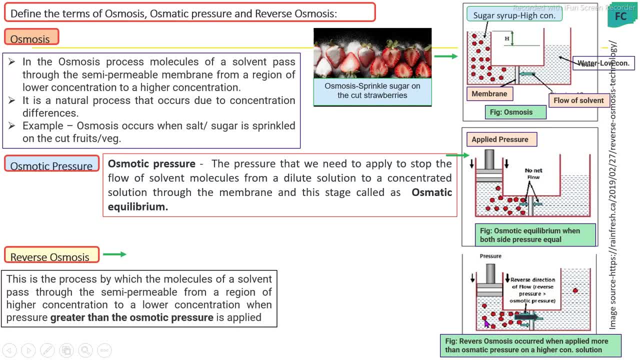 osmotic pressure, in that case the solvent, which is moving from high concentration to low concentration, and this process is called as a reverse osmosis. in the reverse osmosis filtration process, by using the semi permeable membrane, we can separate or the remove the feed material containing. 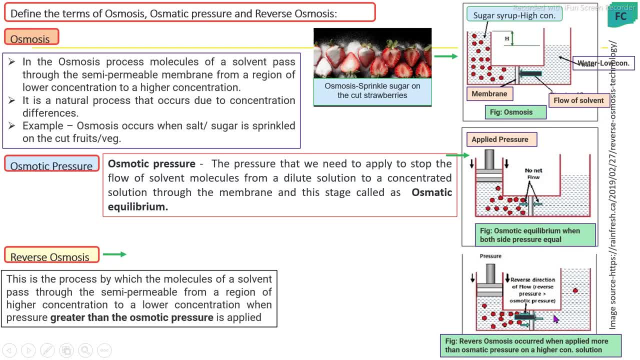 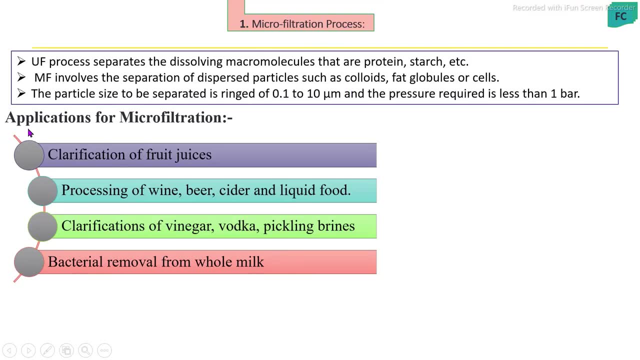 solvent. this solvent is moving from high concentration to low concentration and this process is called as a reverse osmosis. mostly reverse osmosis process is used for the preparation of the concentrated product, the application of the microfiltration. the mostly microfiltration is used in food processing industry for the 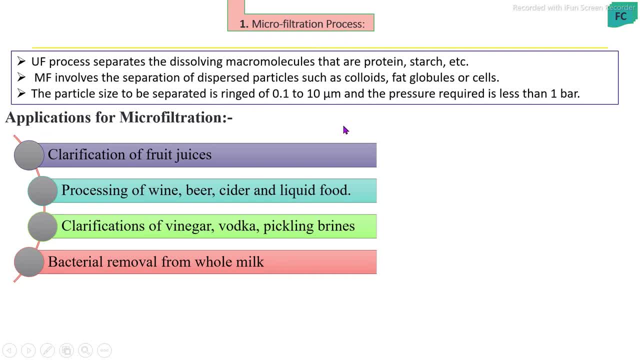 clarification process. what are the liquid foods? is liquid food containing colloidal particles or the dissolved particles, microglial? these are the separated and prepared, the clarified, like the fruit juice, wine, beer, cedars. liquid foods may have clarification of the vinegar, then some of the alcoholic beverages, the 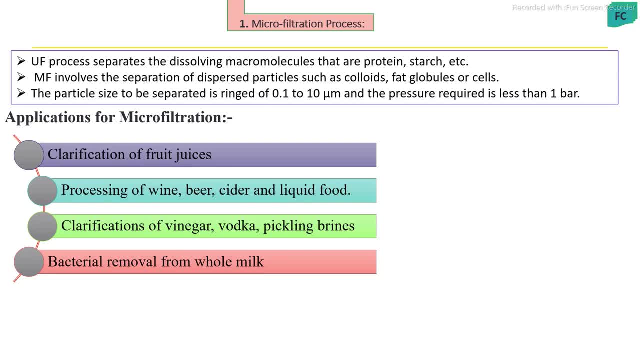 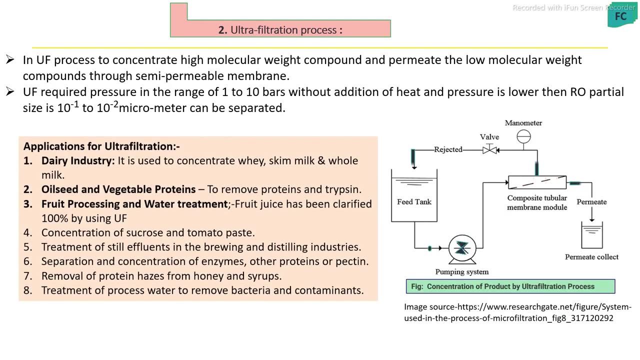 during the preparation of the brine syrups or removal of the microbial from the whole milk. we liquid foods. these are the clarified by the micropigmentation process. the next second ultrafiltration application in the food processing industry. the application of the ultrafiltration reverse osmosis mostly. 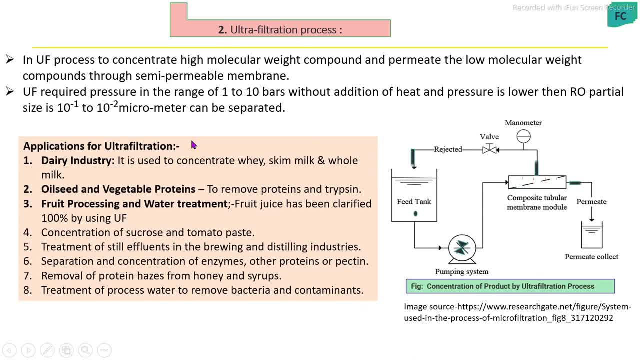 for the preparation of the concentrated product. you can see the application of the ultrafiltration in dairy processing industry for the preparation of the concentrated way: skim milk, whole milk. we can convert this skim milk and whole milk up to 7 to 8- 8 fold concentrated product for the separation of the trypsin inhibitor from. 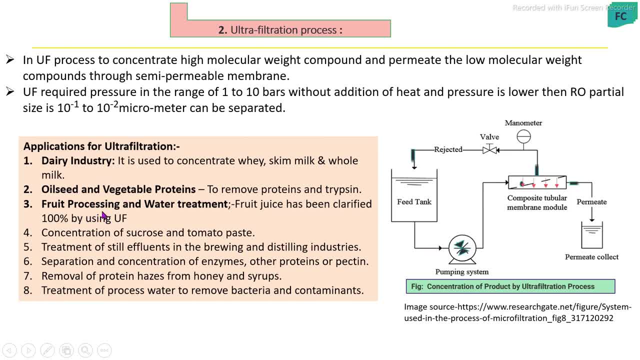 the visitable oil in the clarification of the fruit juices, water treatment and mostly for the preparation of the concentrated product in the enzyme processing technology. these are the main application of the ultrafiltration process in the food processing industry. you can see the simplest example of the ultrafiltration system in the cross flow filtration. 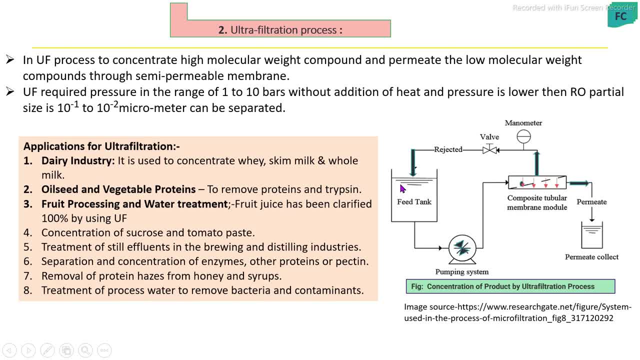 system in the batch, in which we can prepare the concentrated product, the feed tank in the pump, the cross flow filtration system in which, after the filtration, the permit is separated and then concentrated, which is the again recycled, and finally we can concentrate the feed material as per our requirement. 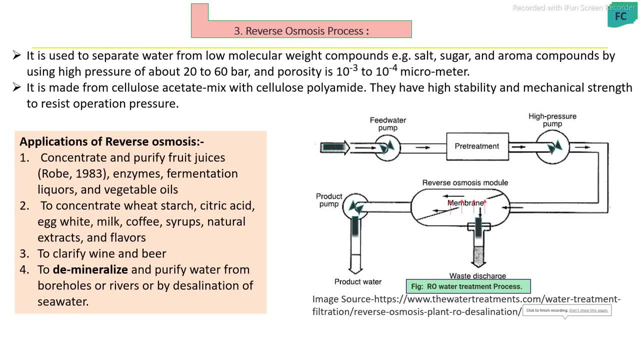 next third one is the reverse osmosis process. the reverse osmosis is basically used for the preparation of the concentrate product- these are the number of the products- and also used for the clarification of the liquid food products in the reverse osmosis, mostly required to pressure related to the initial feed concentration. 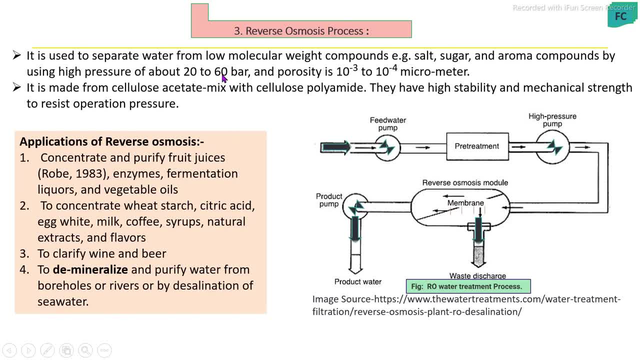 its osmotic pressure, the pressure more than the 20 bar. you can see the simplest example in which the reverse osmosis process: first water, which is the first pre-treatments carried out, in which the pre filters, then micro filters, then number of other filters. these are the pre-treatments process. 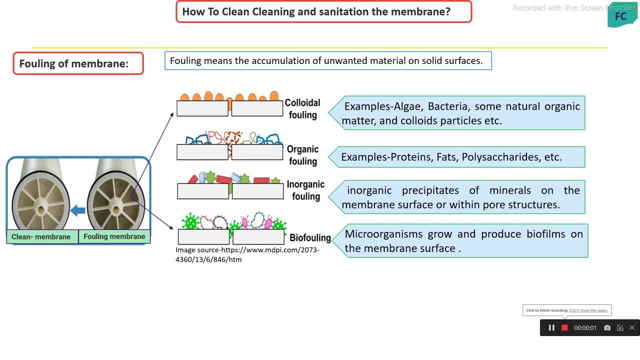 and after that they are the pass into the membrane separation technique, then membrane cleaning and the sanitation process. during the membrane filtration process. you can see in between the processing, the feed containing. these are the number of the matters in which organic, inorganic and provider and biofoiling materials. 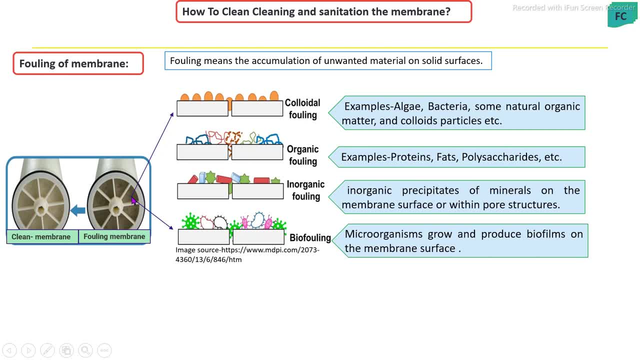 which are accumulated on the surface of the membrane and resulting falling of the membrane. that means in which the these particles which are the formation of the thin layer on the surface, or maybe these particles are blockage the porosity of the membrane. this must require to clean. 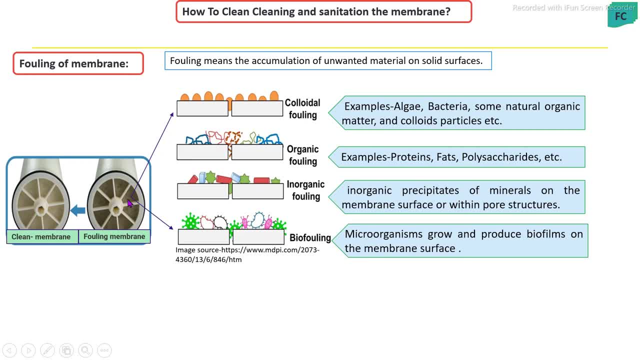 between the processing this falling particles which are the removed by the different techniques. basically, these falling particles are classified into four groups. first one is colloidal particles, in which the colloidal particles including microbial loads and the organic matters in the colloidal form. second, organic matter, in which food constituents, fat, fluid in carbohydrate, like material.